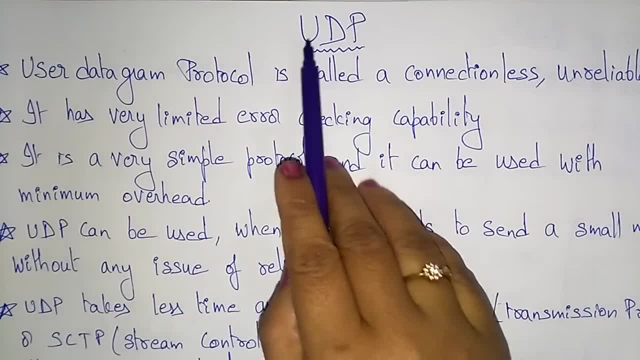 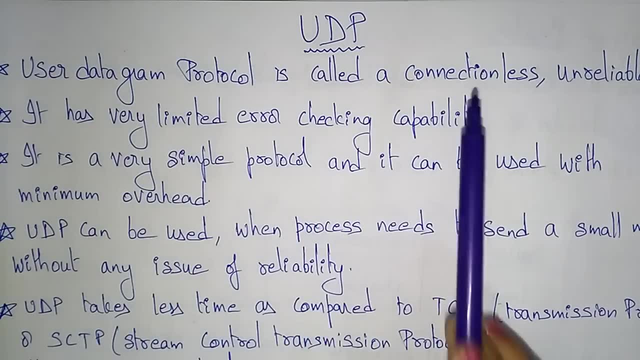 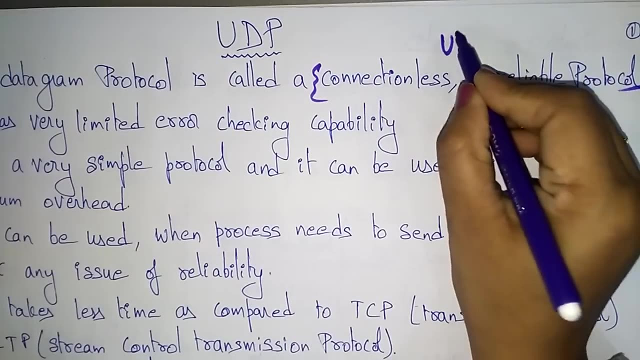 user datagram protocol. We call it as a UDP. U means user datagram protocol. This user datagram protocol is called a connectionless, unreliable protocol. So this point you have to be remember that Whenever you are seeing that UDP, user datagram protocol, means it is a connectionless. 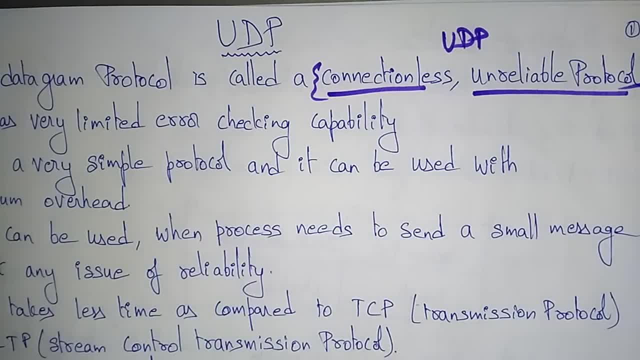 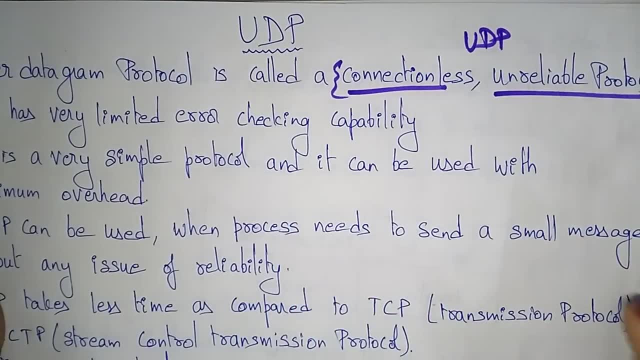 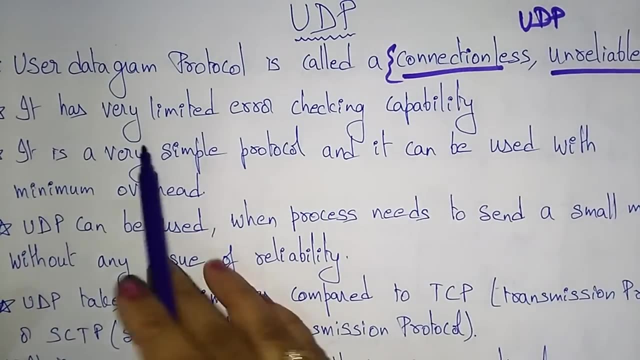 and unreliable protocol. Okay, whereas TCP protocol is a connection oriented and UDP is a connectionless unreliable protocol. It has a very limited error checking capability. So that's why we call it as an unreliable, Because it is only having the limited error checking capability when compared to the TCP. 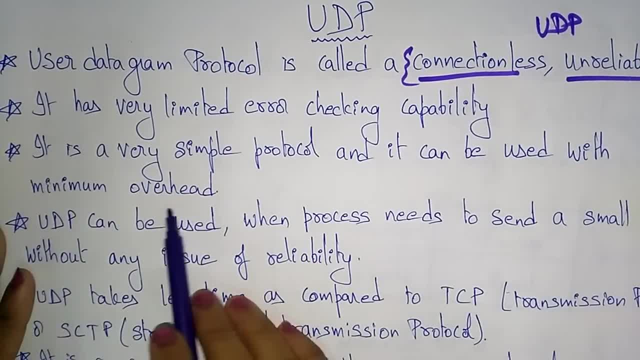 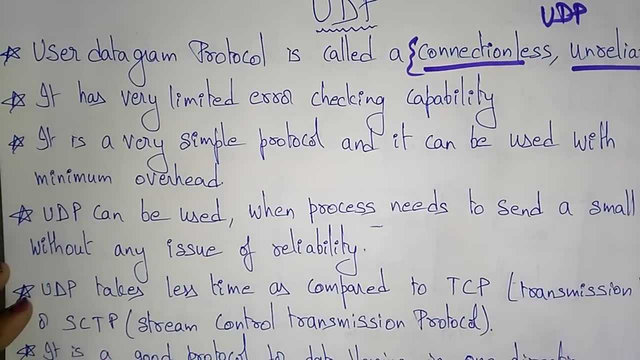 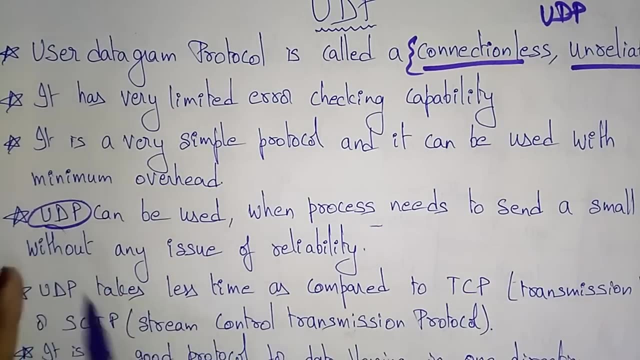 It is a very simple protocol and it can be used with minimum overheads. And user datagram protocol can be used when process need to send a small message without any issues of reliability, So in that cases only you can use the UDP protocol. When we use this UDP protocol, when the process 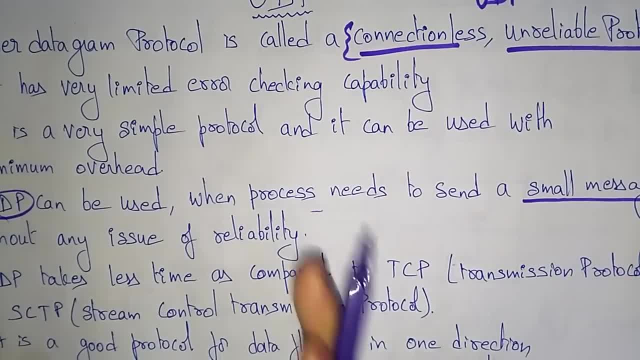 needs to send a small message. So when the UDP is giving small message and the process sent small message Whenever, whenever the transport layer wants to send up message from one process to another processor, Okay, whenever it is sending the small message, then it can go for the UDP protocol rather than. 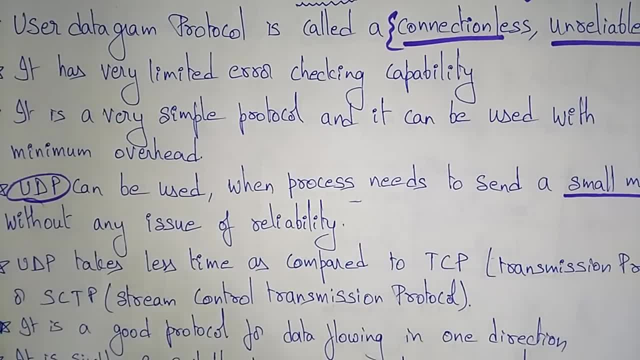 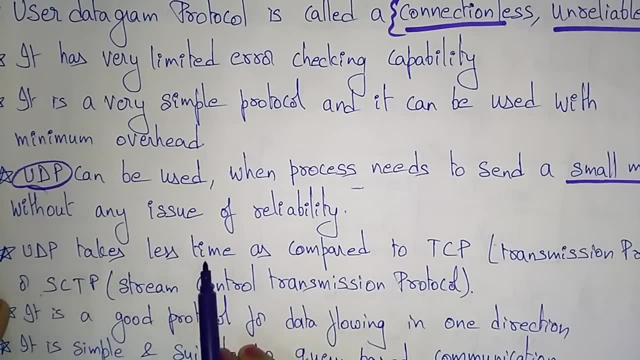 going for the other protocols, So then it can send the message successfully without any issues of reliability. UDP takes less time as compared to TCP. Why it is take less time? only the small messages. that too, without any issue of reliability, so that it takes less. 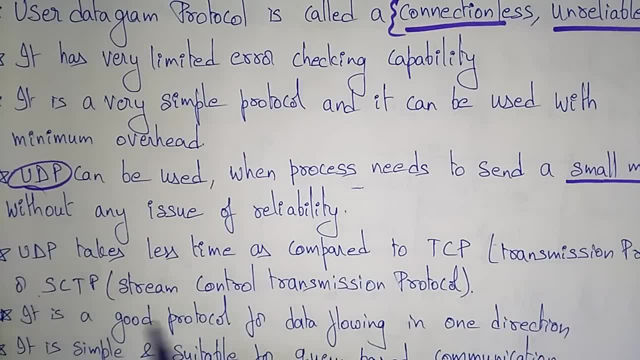 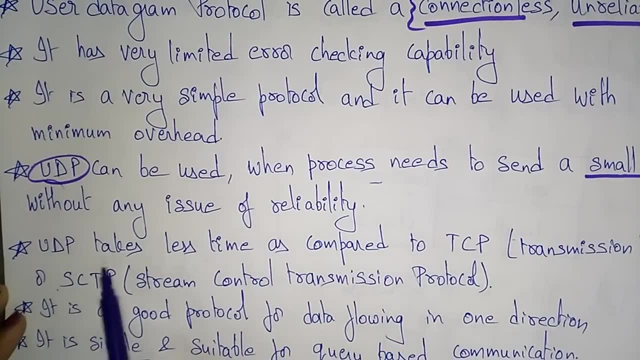 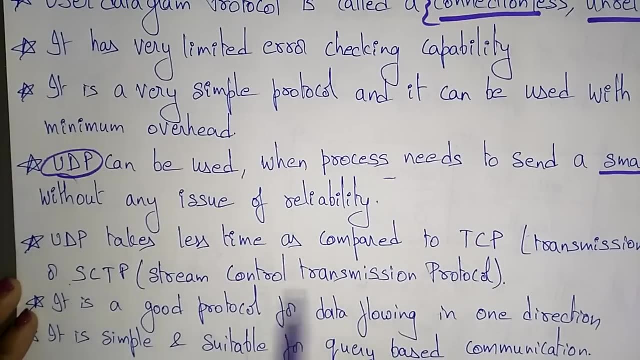 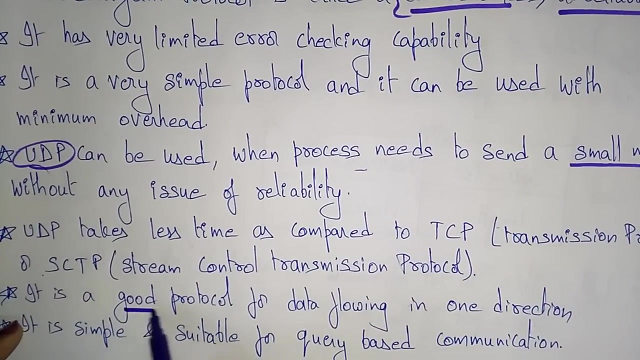 time when compared to the TCP or SCTP means stream control transmission protocol. User datagram protocol takes less time as compared to the transmission control protocol or stream control transmission protocol. UDP is a good protocol for data flowing in one direction, So we call it as a good protocol when we call it as a good protocol whenever the data flowing. 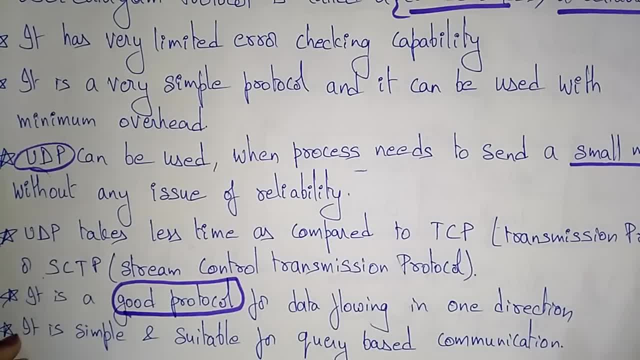 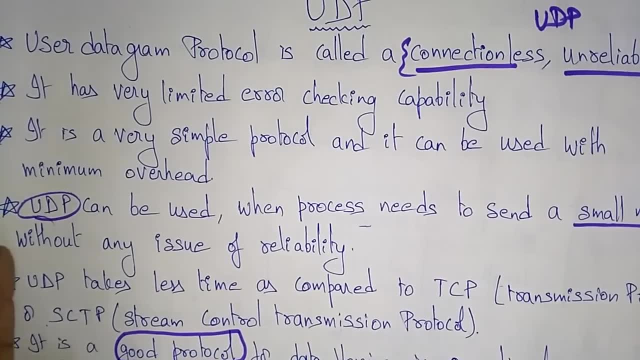 is done using in only one direction, then UDP protocol is a good protocol. It is simple and suitable for query based communication. So these are all the features of the user datagram protocol. Now let us see the user datagram header how it looks like. 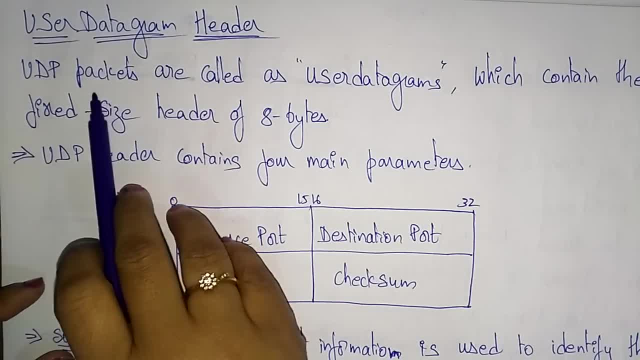 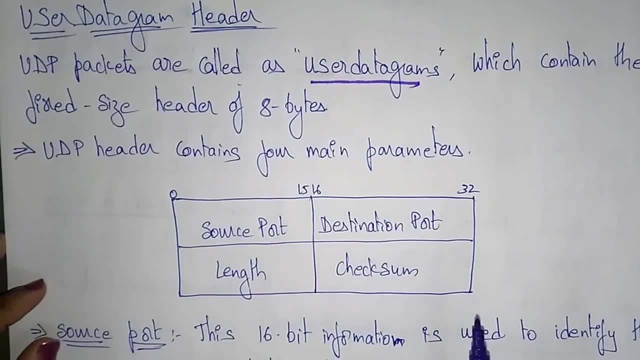 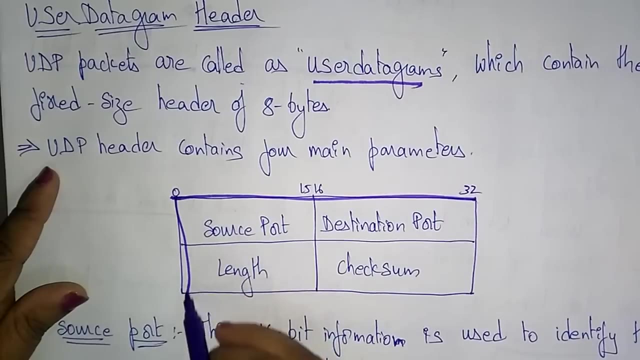 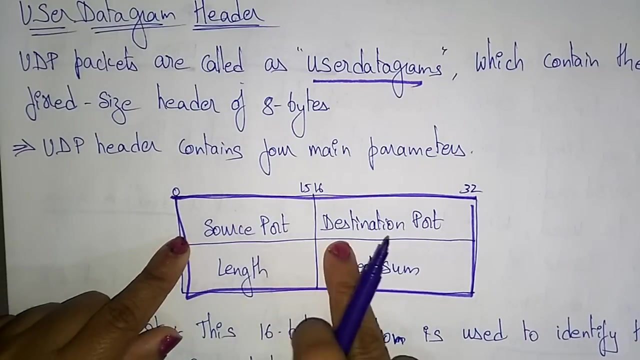 User datagram packet. protocol Packets are called as user datagrams, So which contains the fixed size header of 8 bytes. So here you can see the UDP header. This is a 32-bit header. A 32-bit header is divided into four main parts: Source part is 16-bit and destination port. 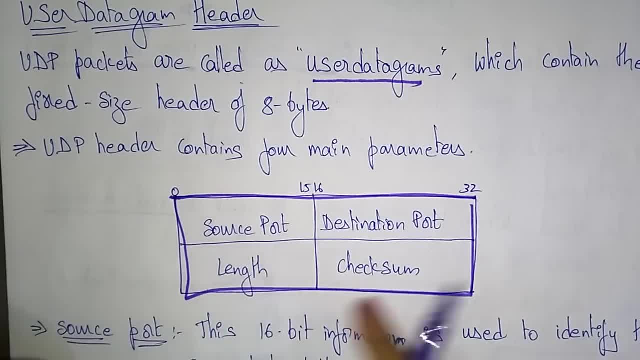 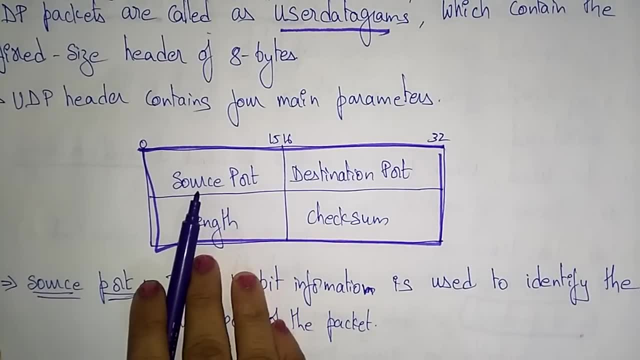 Source port is 16-bit, destination port is 16-bit, length 16, checksum is 16.. So four main parameters. So what is a source port? This is a 16-bit. information is used to identify the source port of the packet. 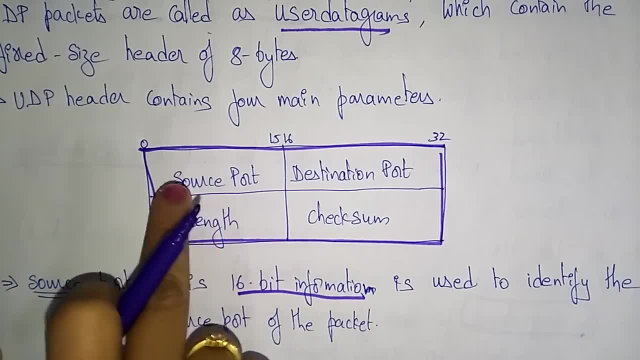 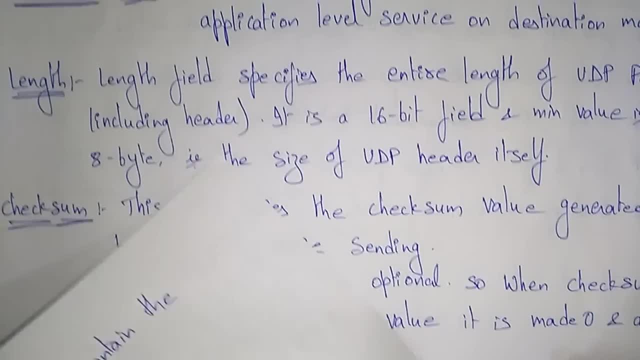 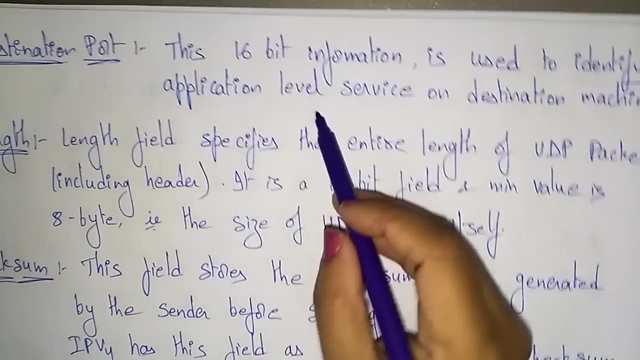 So, whatever the 16-bit information is present in the source port, it is going to be identified the source port of the packet. Then what about the destination port? The next field is destination port. So it is a 16-bit information is used here to identify the application level service on destination machine. 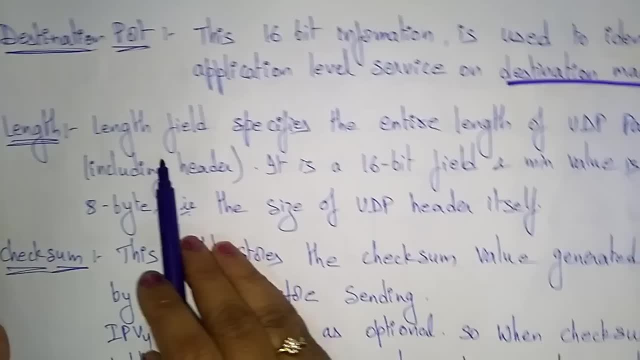 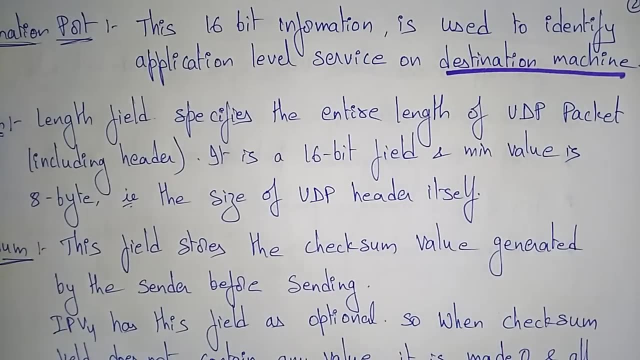 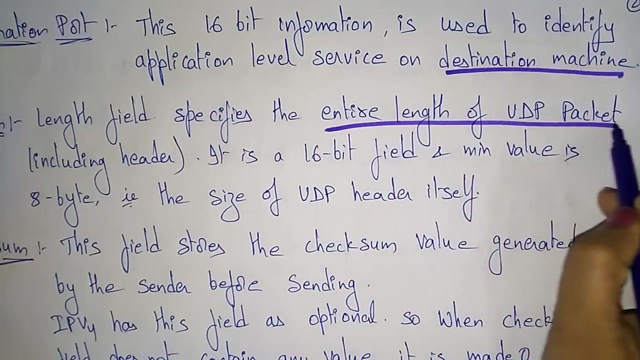 And the next parameter is a web length. The length field specifies the entire length of the UDP packet. So, wherever the in the header format, if you are taking the total length or the length, the length is specifying the entire length of the protocol. whatever the protocol you are taking, if it is a UDP or if it 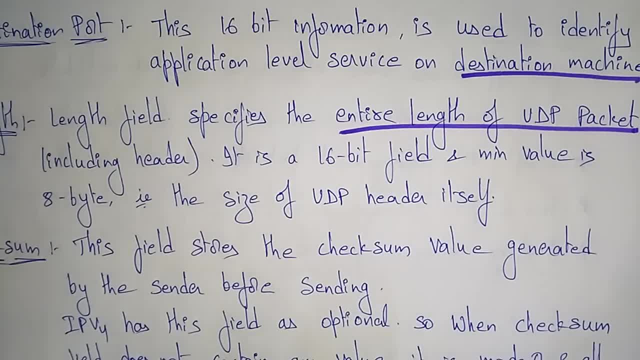 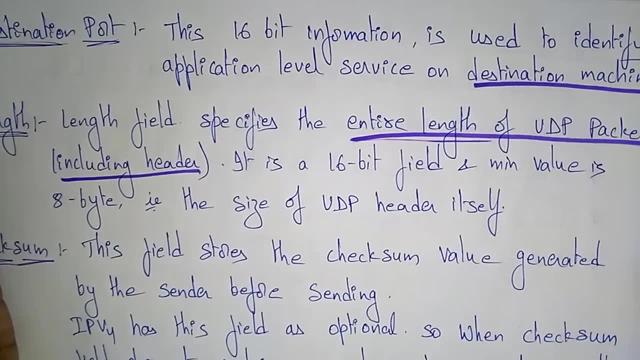 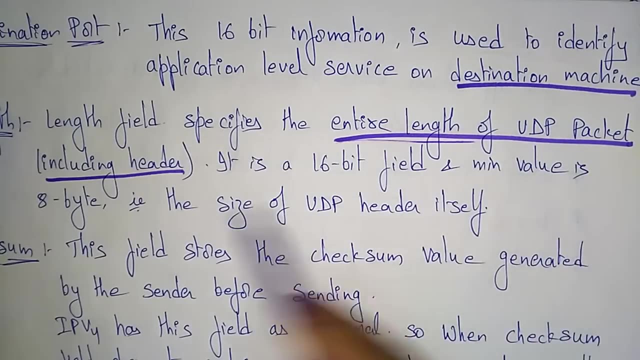 is an IPV, whatever you are taking. So that length specifies the entire length of that protocol. Entire length is nothing, but it is including the header as well as the data. The length field specifies the entire length of UDP packet. It is a 16-bit field and minimum value is 8 byte. That. 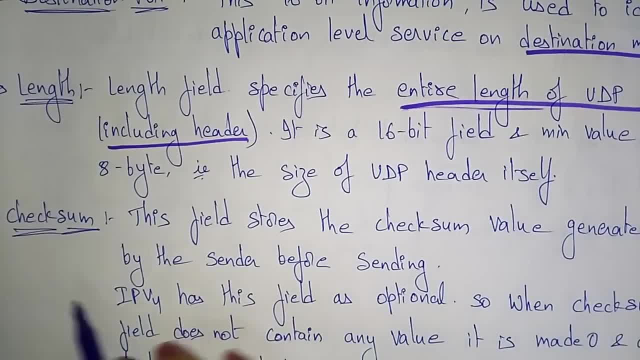 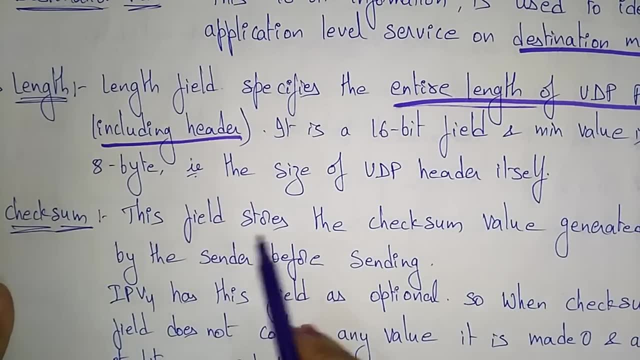 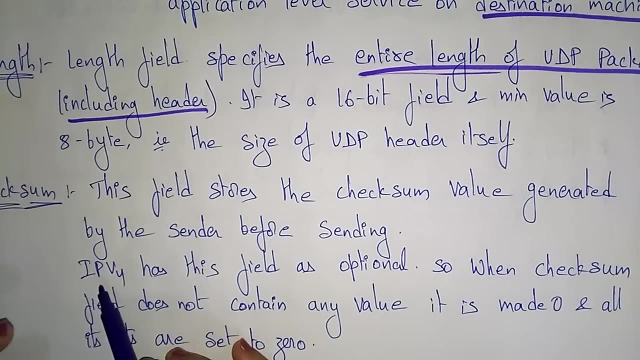 is the size of the header itself. And the last one, next last parameter, is the checksum. What is the use of this checksum? This field stores the checksum value generated by the sender before sending. So here, IPv4.. The internet protocol version four has this field as optional. So if you just seen that IPV version.